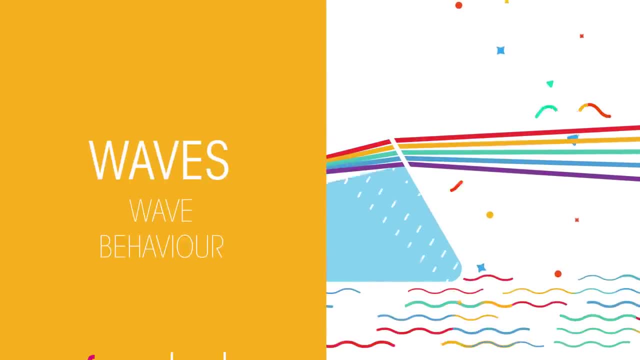 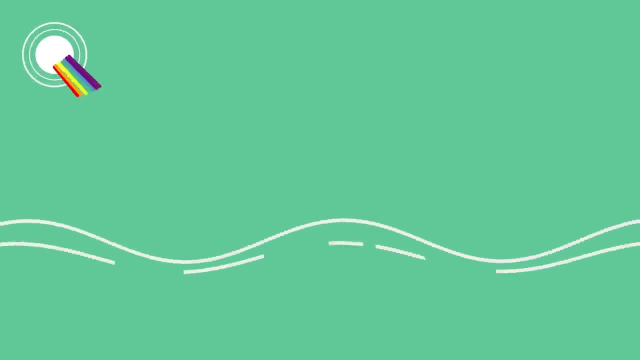 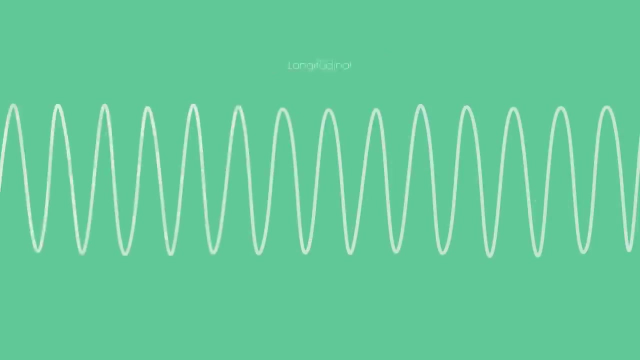 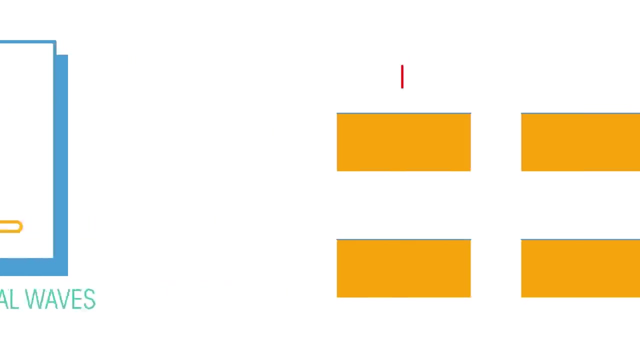 How do waves behave Badly. In this video we're going to look at how light and sound waves behave. Before we start, you should know that waves can be transverse or longitudinal. To learn more about the properties of waves, watch this video first. Transmission, reflection, refraction, diffraction. 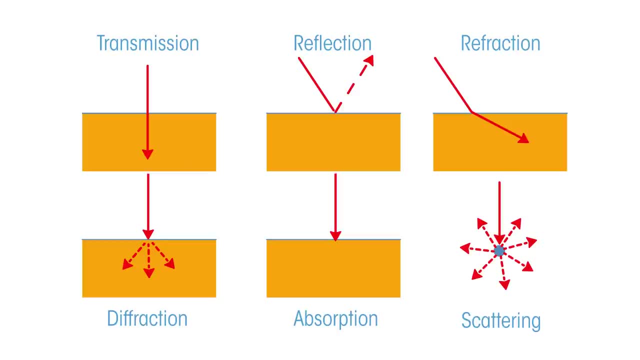 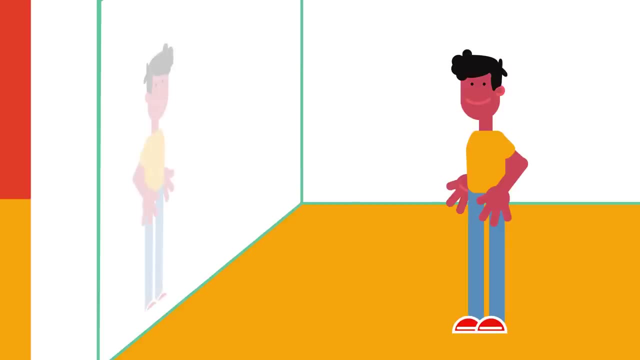 absorption and scattering are all typical wave behaviors. Reflection is when waves bounce off an object. Sound waves are reflected by hard, flat surfaces and is why we get echoes. You hear a delay between the original sound and the echo because the echoed sound waves have to travel. 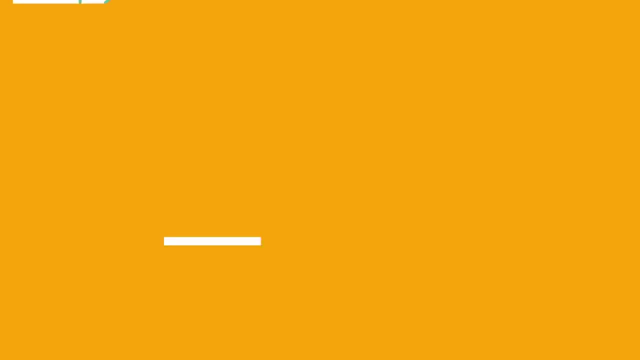 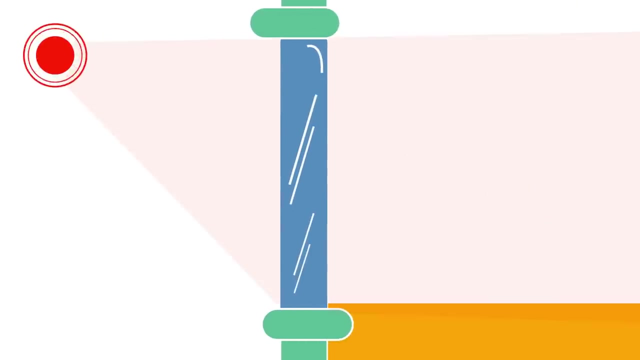 twice as far to reach your ears. Smooth surfaces like glass or polished metal reflect light in a regular way, so a reflection can be seen like a mirror or seeing your face in a calm pond. Transmission is when waves keep travelling in the same direction through an object like light. 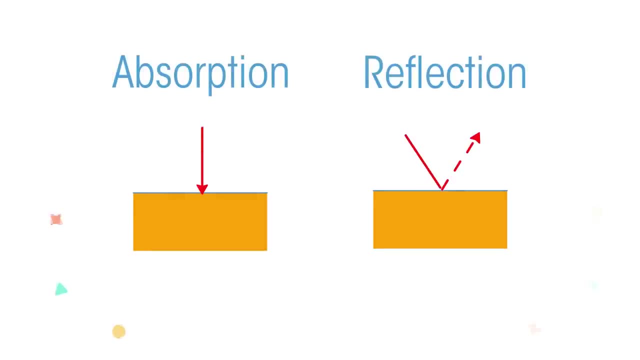 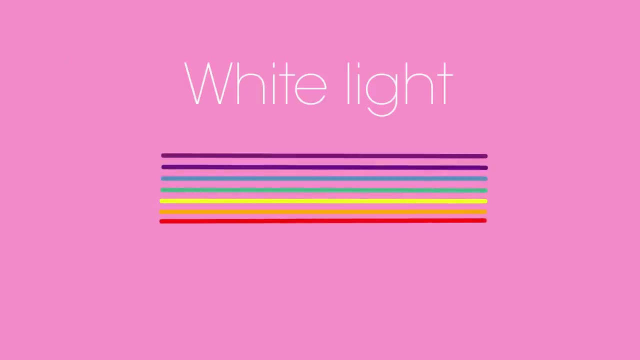 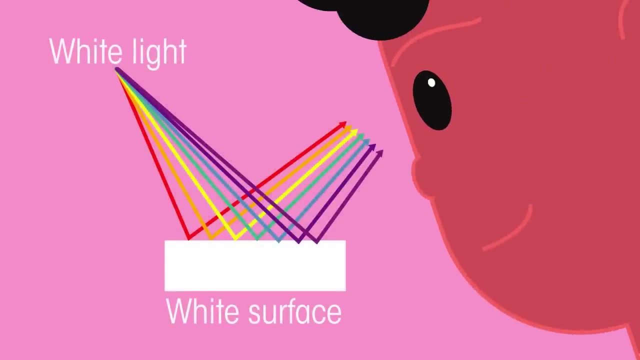 through a window. Absorption and reflection often go hand in hand for light waves. White light contains each wavelength, so all the colors of visible light. The colour of an object depends on which wavelengths of light it absorbs and which it reflects. White objects reflect all the light that hits them and absorbs none. 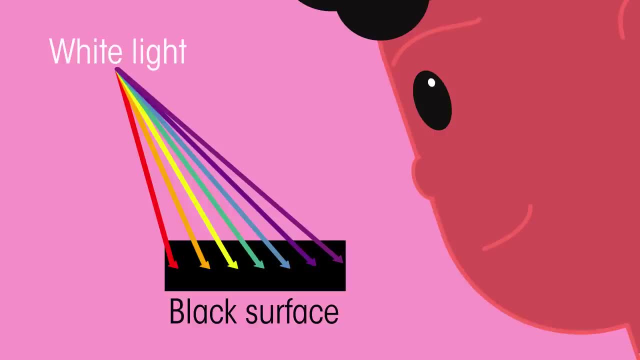 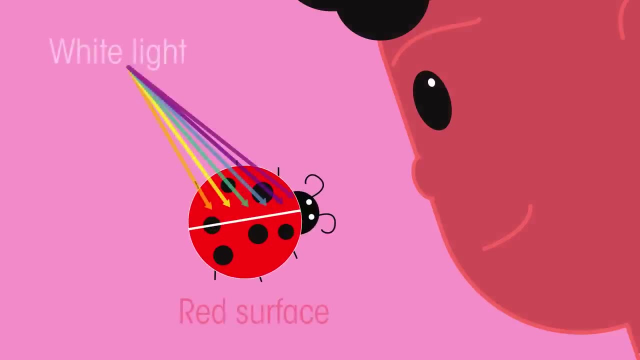 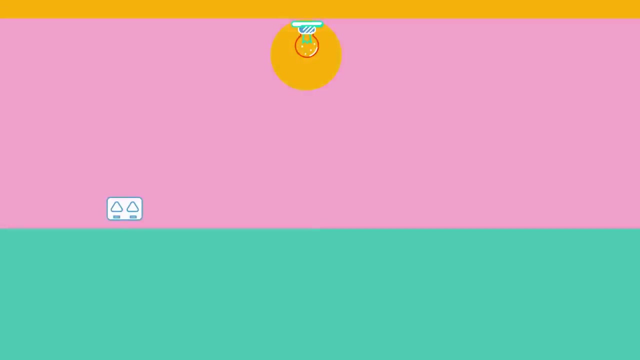 Black objects reflect none and instead absorb all the light that hits them. A red object absorbs all the wavelengths except the red, which is reflected, And a green object absorbs all the wavelengths except the green which is reflected. Are the new people upstairs really noisy? 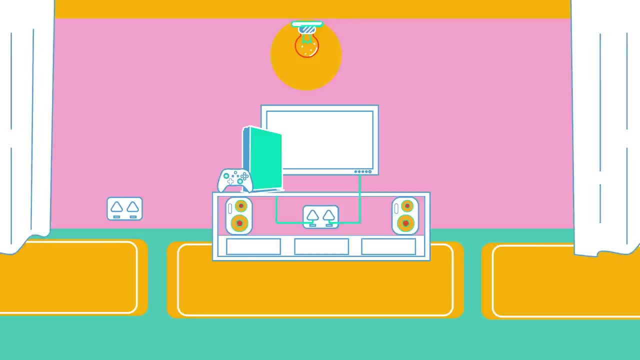 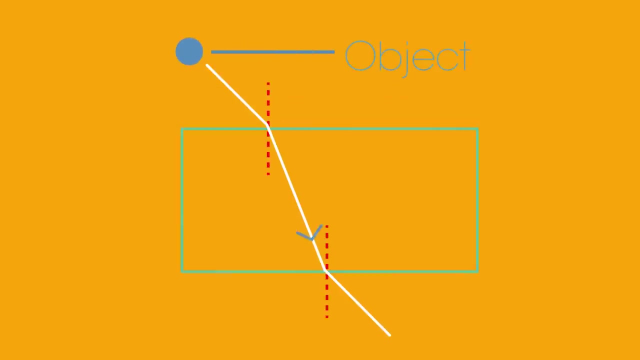 If they carpet their floors, add curtains and furniture to the room, then you'll notice that they'll become much quieter. This is because some objects absorb sound waves. When someone is in a room, the sound and light waves pass across a boundary between two substances. 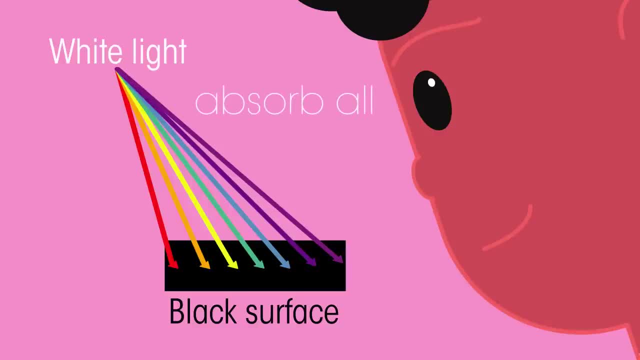 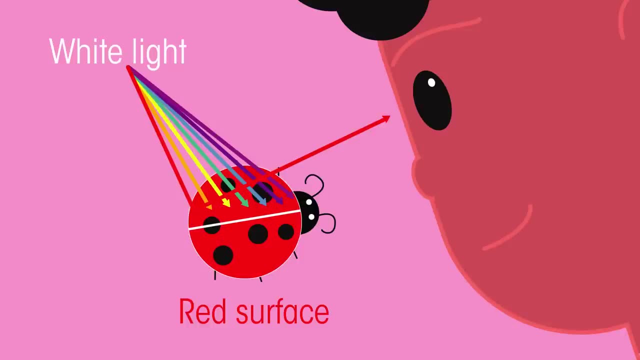 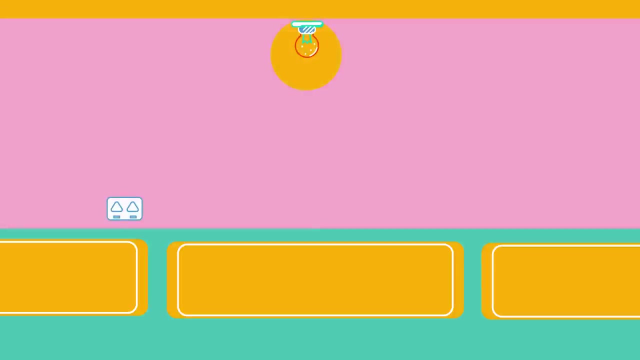 instead absorb all the light that hits them. A red object absorbs all the wavelengths except the red, which is reflected, And a green object absorbs all the wavelengths except the green, which is reflected. Are the new people upstairs really noisy If they carpet their floors? 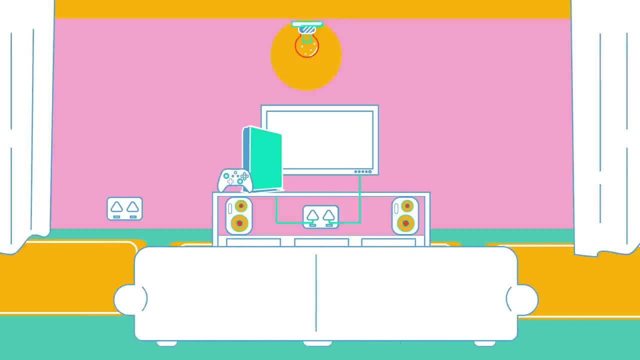 add curtains and furniture to the room, then you'll notice that they'll become much quieter. This is because some objects absorb sound waves. When sound and light waves pass across a boundary between two sides of the room, they are called sound waves. When sound and light waves pass across a boundary, 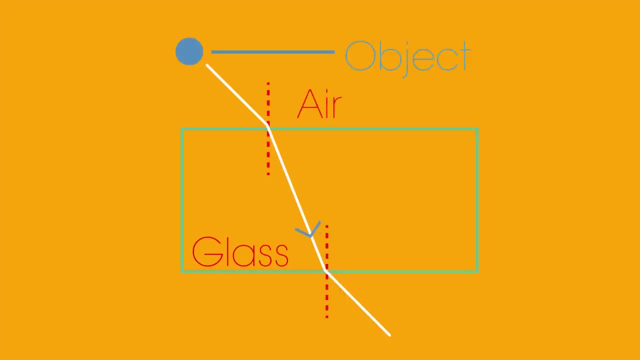 between two sides of the room. they are called sound waves. Like air and glass, they change speed. This is because the substances have different densities. The change in speed causes the waves to change direction, which is known as refraction. Because of refraction, things in water look closer than they really are. 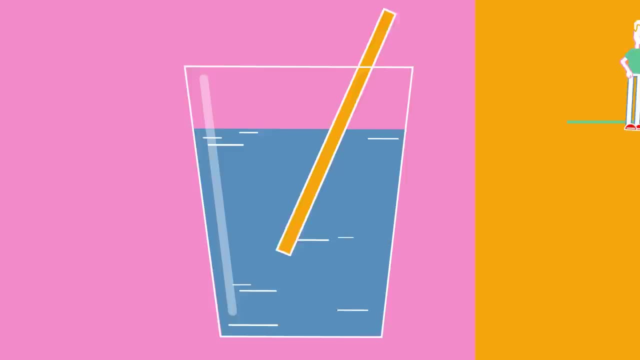 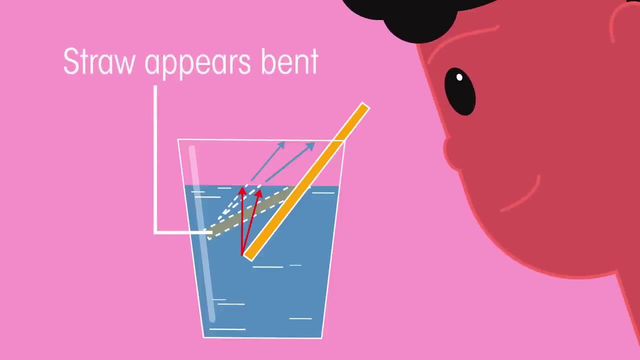 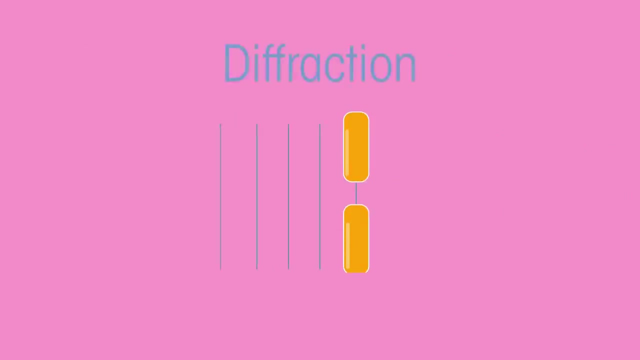 Water appears shallower than it really is And a straw in a glass of water looks like it bends at the surface Because the refracted light wavelengths make you think the straw is in a different place to where it actually is. When waves meet a gap in a barrier, they pass through the gap. 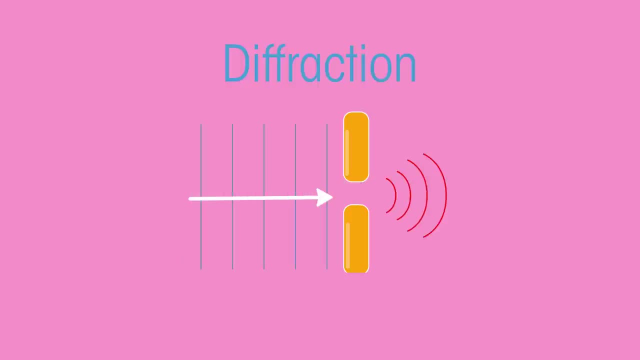 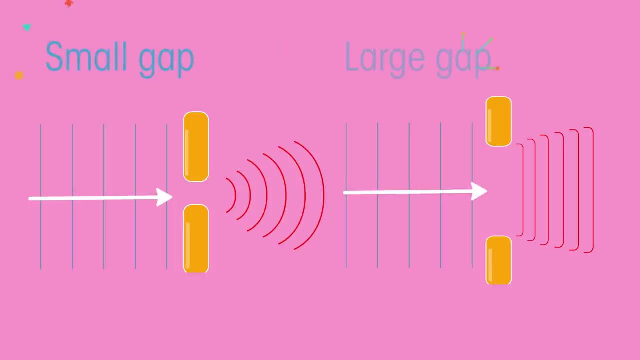 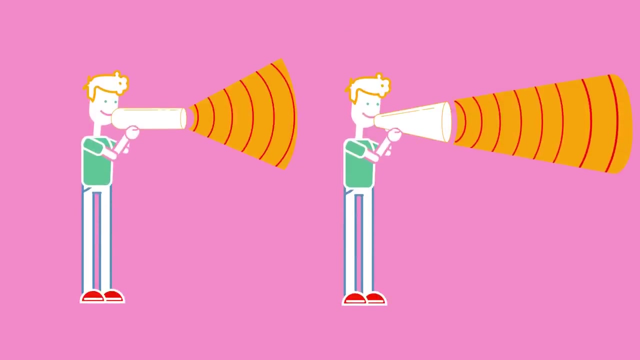 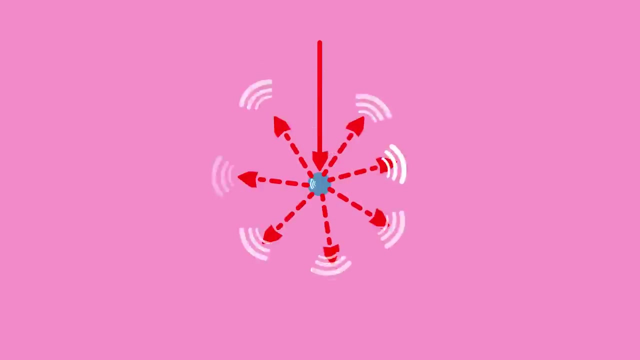 They then spread back out after they pass through the gap. This is defraction. The way the waves re-spread depends upon how big the gap is compared to the incoming wavelengths. We have diffraction to thank for loudspeakers. Sometimes waves depart from the expected path and spread out in multiple directions. 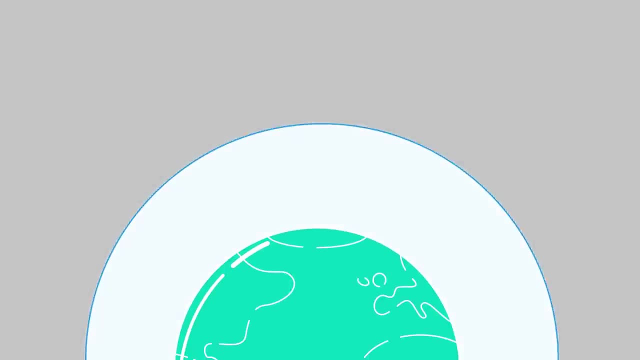 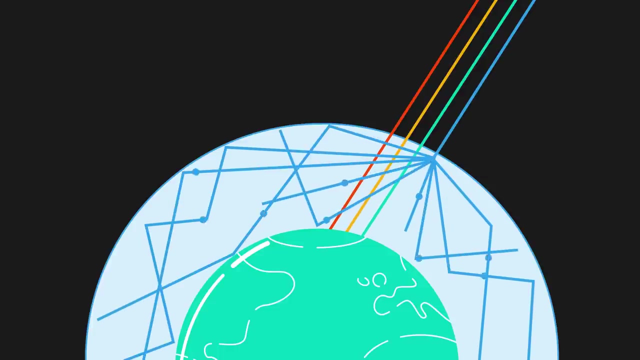 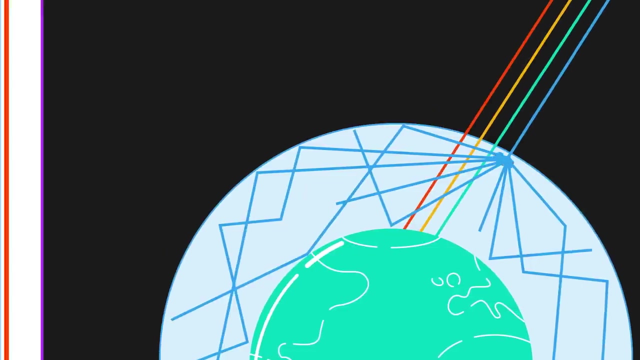 This is known as scattering. We have scattering to thank for making the sky appear to be blue. The white light coming from the sun hits the molecules in our atmosphere, which causes the shorter blue wavelengths to scatter out in all directions And the material emits is called light. 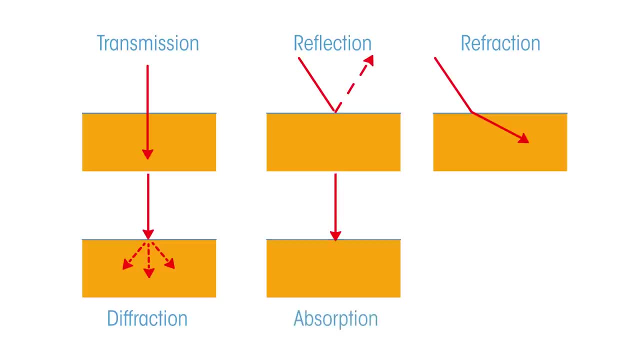 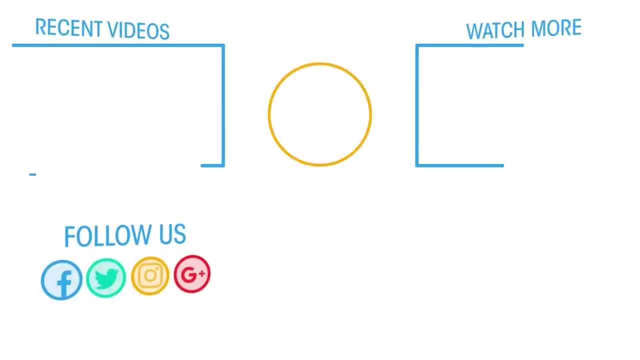 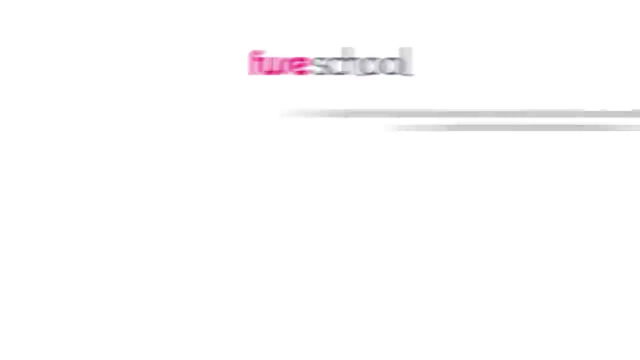 So waves behave in a variety of ways depending upon what material they hit. As such, the information you watch on the screen is not the correct answer. This video does not completely reflect the actual events of the recent tidal waves. This video does not reflect the actual events of the previous eight matter wavelengths. but it does reflect the current events, of the current auditory movements as well as other phenomena. This video also contains some information about the existence of the center of the Milky Way, the Earth, the cosmos and even the entire galaxy. This video is not completely correct. If this video is correct, then it means the video is correct.